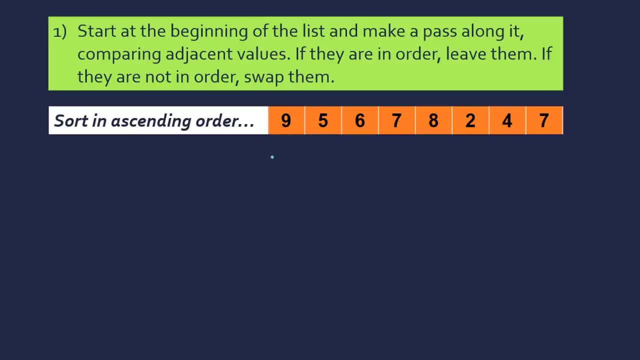 nine and five. Are they in order? Well, they're not, because we need to swap them, because it needs to be ascending order. So we basically will just write down nine and five And I'm not going to write out the rest of the list each time, because that game is a bit of a. 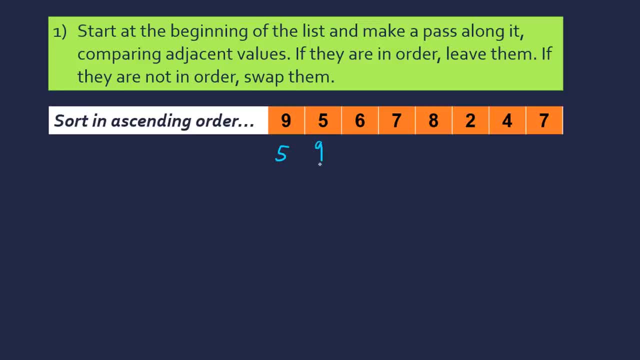 waste of time. So what you can next do you now? you now. nine is now in the second position, So you now compare nine with six. Six is also less than nine, So you swap them. You now then compare nine and seven. Seven is less than nine, So you swap them. Nine and eight. 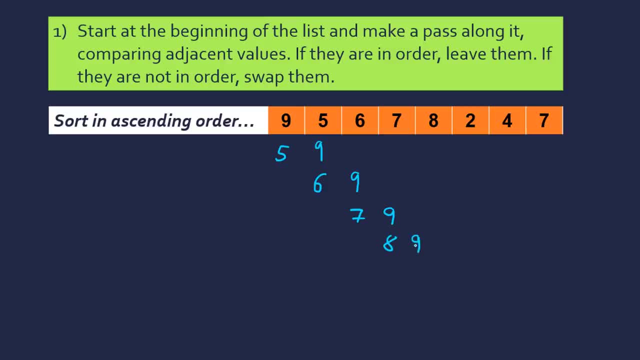 Eight is less than nine. So we can see- I've deliberately done something here- So you can see nine essentially bubbling towards the end, as I say earlier. So nine again is greater than two. So two nine is roughly in line. Four is less than. 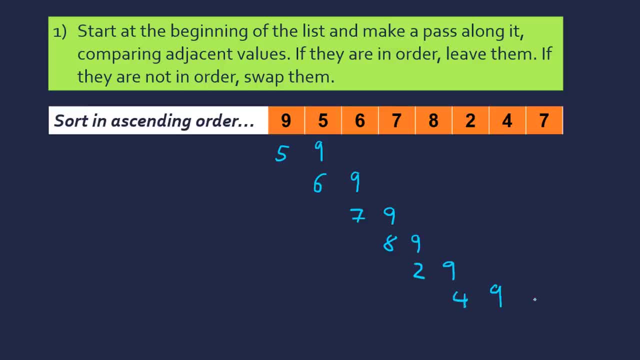 nine, And nine is greater than seven. So nine bubbles towards the end, And again, you could write out the rest of the list each time, but you don't really need to to see what's happening. So nine bubbles towards the end, And now you can leave nine in the next pass. This is only. 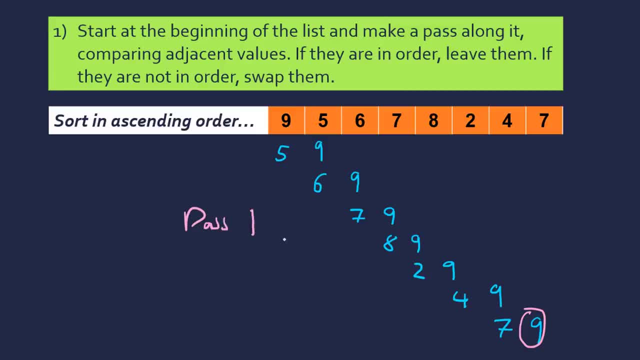 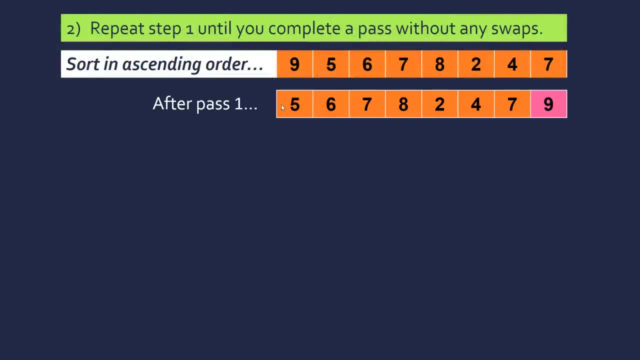 one pass. This is our first pass at this problem And nine is now sort of sorted. So nine is the largest of the list and it's bubbled towards the end. Okay, to spare you my handwriting, here's our result from the first pass. So nine is sort of sorted already. It's almost. 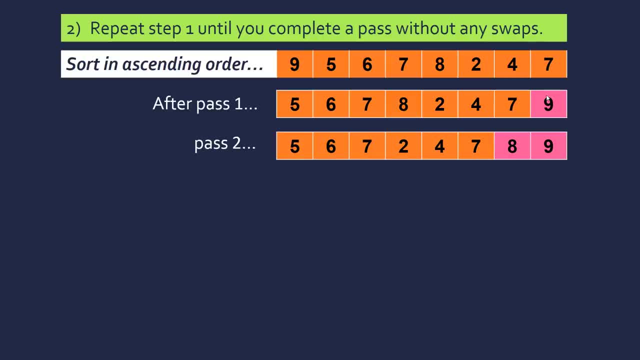 like it's a partition within the list. So after the second pass, eight bubbles towards the end, It's the second largest. So now these are kind of separate. After the third pass, seven bubbles towards the end, You've got two sevens, which doesn't make too much difference actually, in sort of a general sense After. 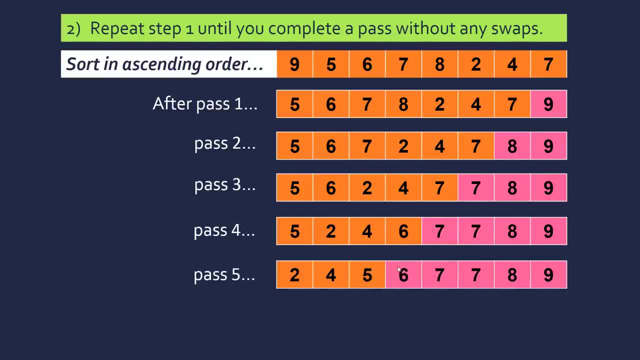 pass four. the other seven is added in this order After pass five, six, And then it's actually all done at this stage, but we have to do a final pass. You've got to remember this is done by a computer. We can notice that this is an order, but a computer has. 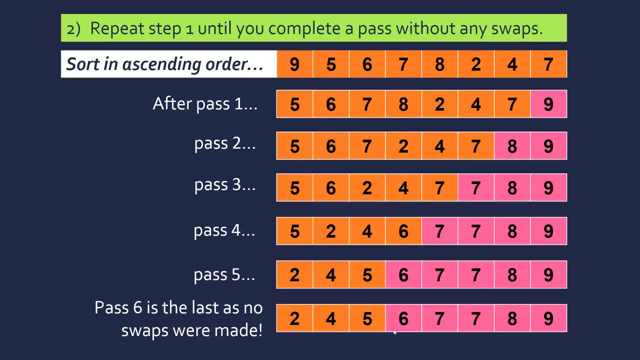 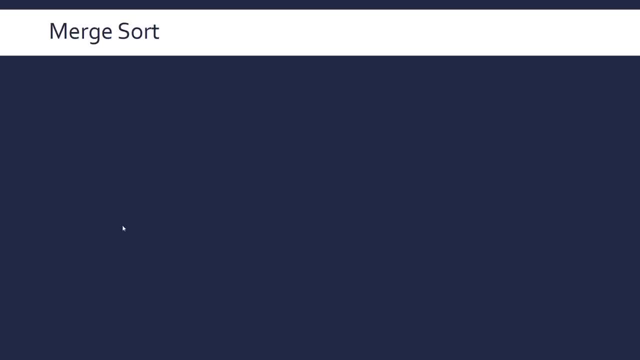 to be sure, And the way it can be sure is it goes through the pass without actually swapping anything. This is how it knows when to terminate, because it's sorted. So this is our final result. Let's now look at a slightly more complicated algorithm, I'm afraid, but a much more useful. 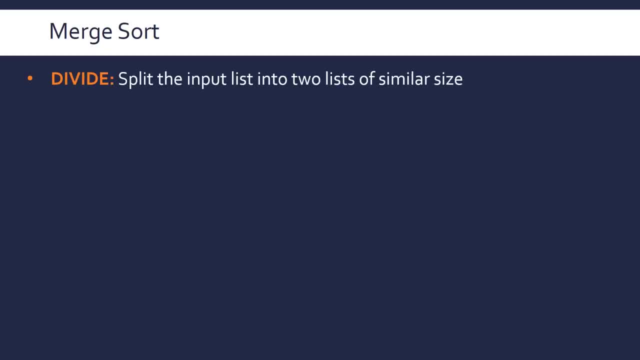 one. It's much more efficient than bubble sort. Merge sort is a divide and conquer algorithm. It's a class of algorithm divide and conquer, And in the divide step the input list is split into two lists of similar size And in the conquer step both sub lists are. 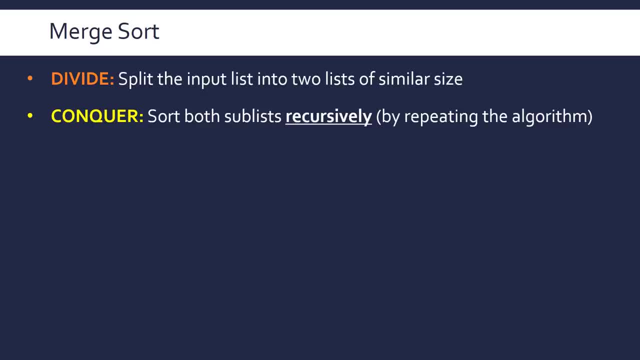 sorted recursively. And recursively means to call the algorithm from within the algorithm, So it's repeating the algorithm for each sub list, which may not make a lot of sense. So you can kind of understand merge sort without knowing how it works recursively, but it's. 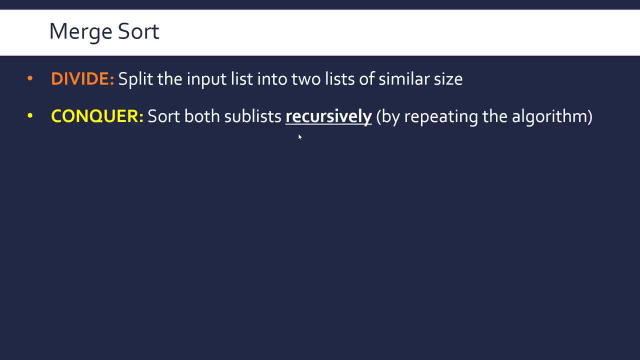 useful to know, because recursive behavior is very common in computer science as you move forward, But ignore it for now- To combine it you then have to merge your sorted sub list into one sorted list, So to kind of go through the algorithm in simpler terms without 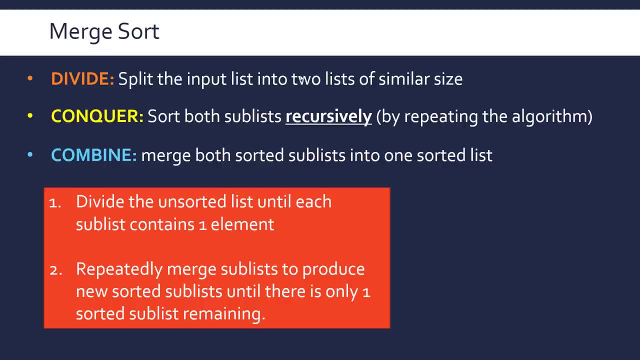 talking about recursion. first of all, you're dividing the list until each sub list contains one element Sub list, Sub list is taken to be sorted because it is effectively sorted. It then has to repeatedly merge these sub lists, these sorted sub lists, to produce new sorted sub lists, until you. 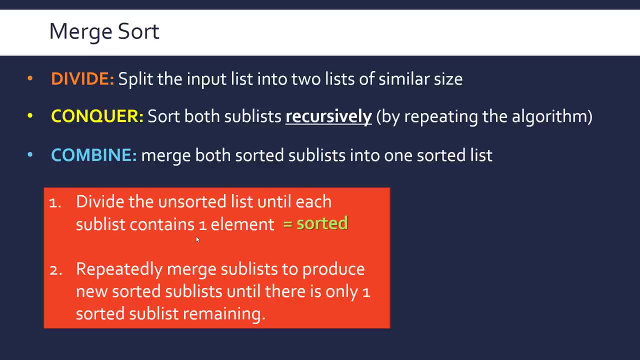 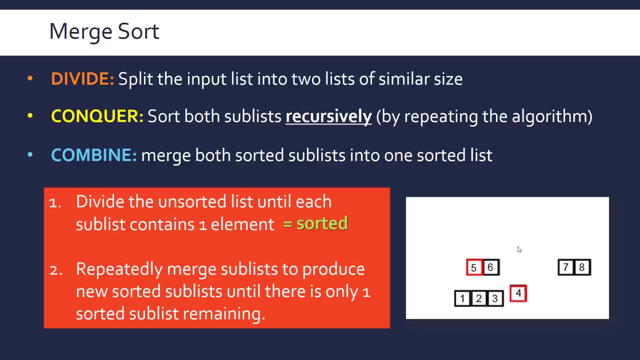 only have one sub list, which is your. well, it's not actually a sub list, it's your output. And this is a GIF which comes from Wikipedia. Wikipedia is quite good for algorithms. actually, It's showing you the merging step now, But we'll show you it. I'll show it myself, So 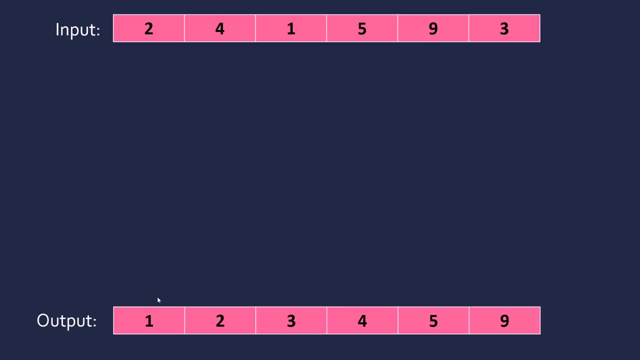 we're going to have our input list here and we're going to end up with our input list. So we're going to have our input list here and we're going to end up with our output here. So the first step is to divide this until we get to a step where each sub list is of 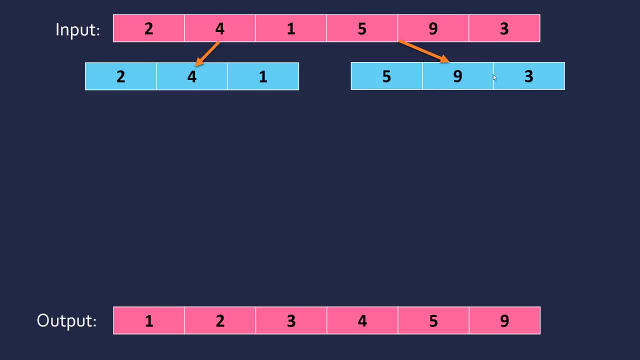 length 1, so it's sorted. So we're dividing this into two equal sized sub lists, not actually doing anything to all of them at this stage, And this is where the recursion comes in at this step So effectively. now the algorithm is calling itself on each sub list, So it 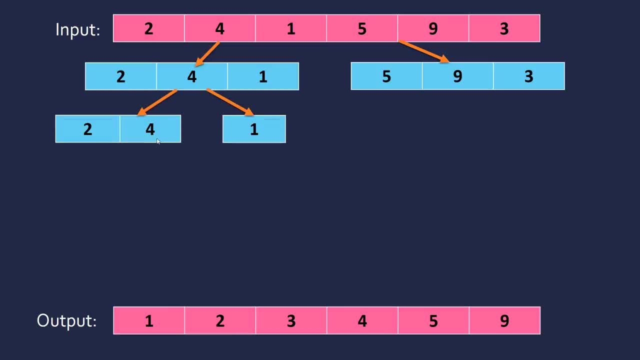 takes 2, 4 and 1 to be the input sub list. So it divides this again into two separate lists. Again, you don't really have to understand the recursion to just know that it keeps splitting it until it gets to size 1, until each sub list is of size 1.. But these are two distinct. 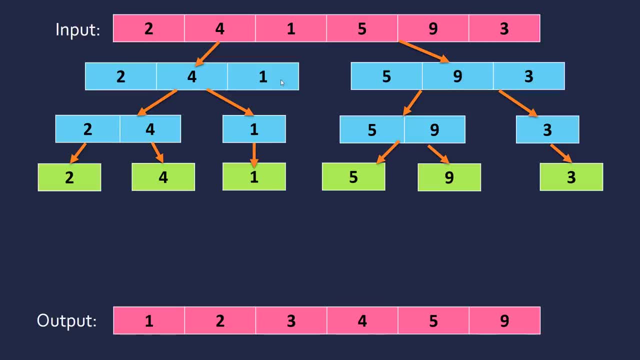 recursion calls. So we've now done the divide step, because each are of size 1.. We're then going to have to actually conquer them and then merge your results. So to conquer we need to sort it in this case. So 2 and 4, I kind of sorted and merged together. 1 and 5 are again in. 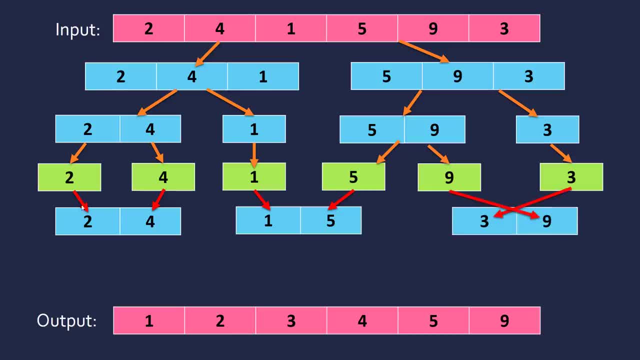 order. so that's fine, But 9 and 3 have to be swapped, and then we have to combine the steps from each of these, So 2 and 4 and 1 and 5.. What it will do, it will do- is it will. 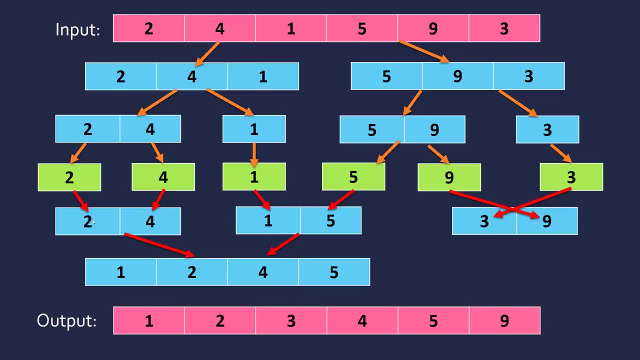 leave an error. I've simply got an error in here. That's what we're going to do here. Okay, so now the steps. These are all the steps and these are the ones I'm going to use, Those. We will look at the two smallest elements and compare them. 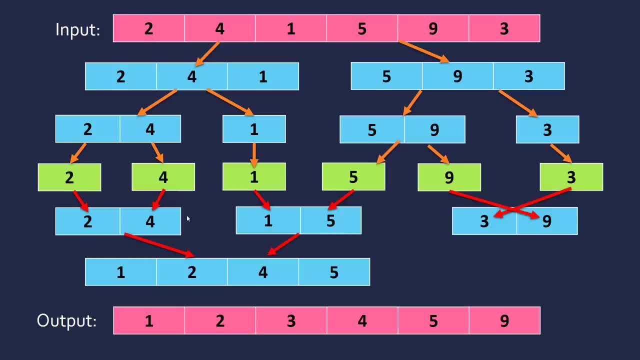 So 1 is less than 2, so 1 goes to the front. 5 is greater than 4, so 5 goes towards the end and 3 and 9 is on its own because we have an odd number. it's slightly awkward. 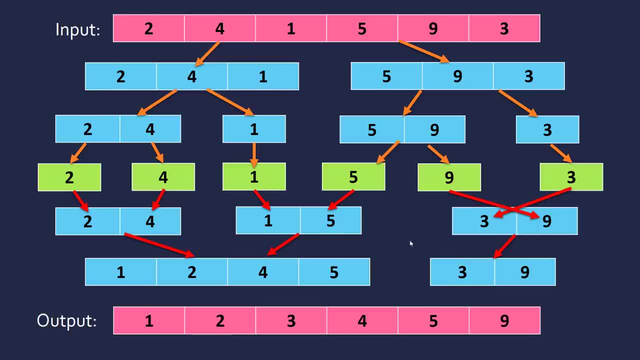 But then we can combine these finally by going: 3 is greater than 1 and greater than 2, so 3 slots in the third position, and 9 is greater than 5, so 9 goes towards the end. So we are dividing it at the first stage and then we are merging them to ensure they are. 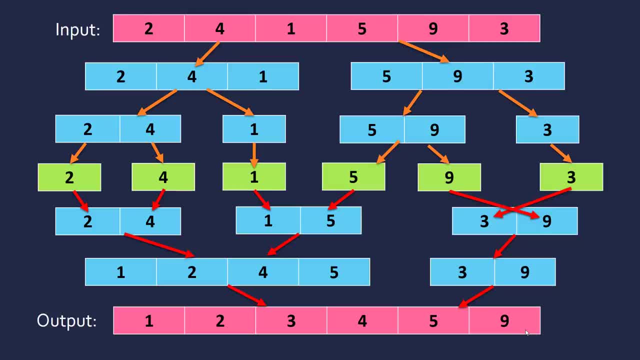 sorted. but it actually works with recursion because it repeats the algorithm for each sub-list effectively. But you don't need to necessarily understand that to know that this is the output we get from using merge sort. A third and final algorithm we are going to look at for sorting is insertion sort. 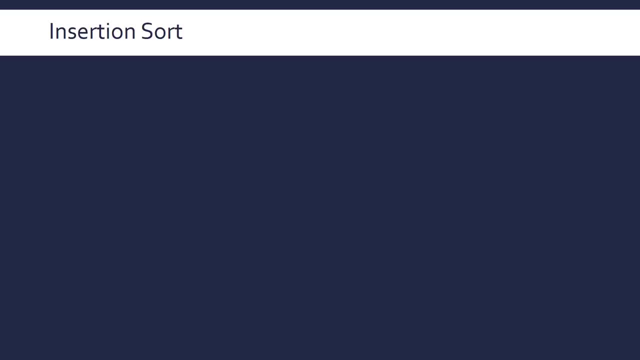 This is simpler than probably both bubble sort and merge sort, thankfully So. what this does is it divides a list into a sorted part and an unsorted part. You can think of it in terms of two separate lists, but in implementation it is certainly done on the same list, with just partitions. 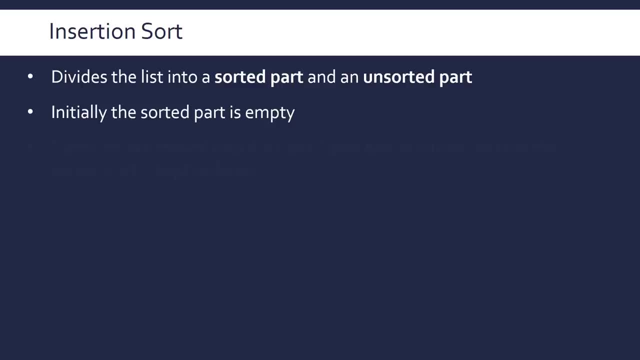 So, initially, your sorted part of the list is empty and then you continually, as you loop through, add an element to that list, ensuring that the sorted part is kept ordered, which will make sense right now. So this is the same list we did, I think, bubble sort with, and we have our sorted bit, which. 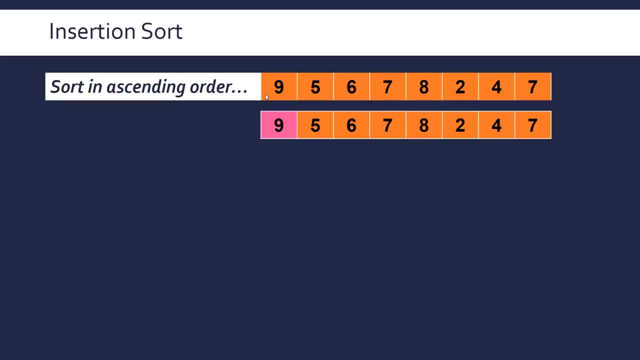 we are going to do in pink. So initially, in the very first step, this is empty, or you can take this to be the first step. it doesn't actually matter. but effectively the sorted list has just got 9 in it now, so it is sorted. 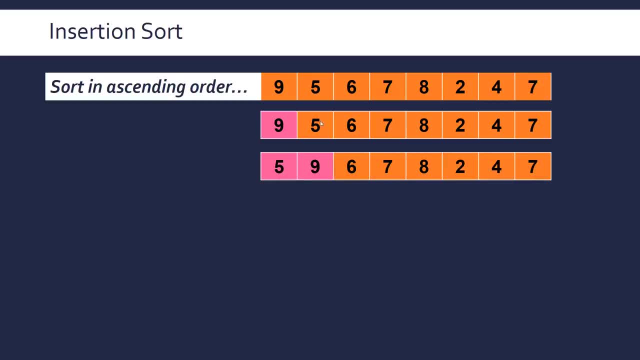 The orange bit is the unsorted part of the list. So we now add 5 to this and we need to keep it in order. so 5 gets put before 9 and they get compared. 5 is at the first position. We then add 6 to the sorted part. 6 is greater than 5 but less than 9, so 6 goes in the middle. 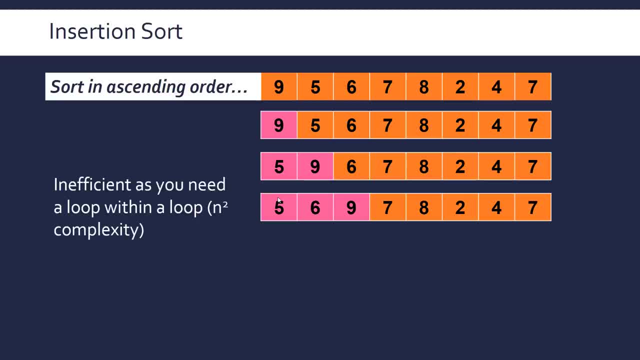 and hopefully you can see now, or some of you might be able to see now, why this isn't a very efficient algorithm because you have kind of nested loops. you've got a loop within a loop, which is very bad for efficiency. Bubble sort is not as obvious that it does this, but bubble sort is the same when you 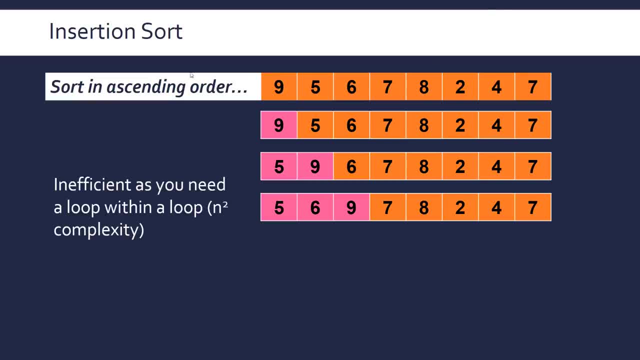 actually implement it. You've got a loop within a loop, Because you're looping across the list in general, but then you're looping within the sorted part of it to put your element in order. So not ideal. This is not very efficient. It's a lot less efficient than merge sort, as we'll talk about in a minute. 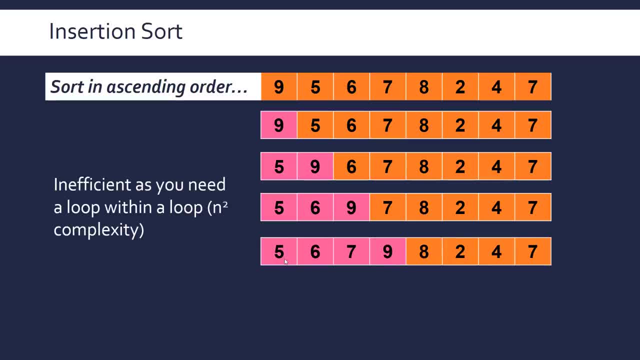 So now we need to add 7 to our sorted partition. 7 is greater than 5, is greater than 6, is less than 9, so 7 goes in that position and we can kind of skip the rest of this now. 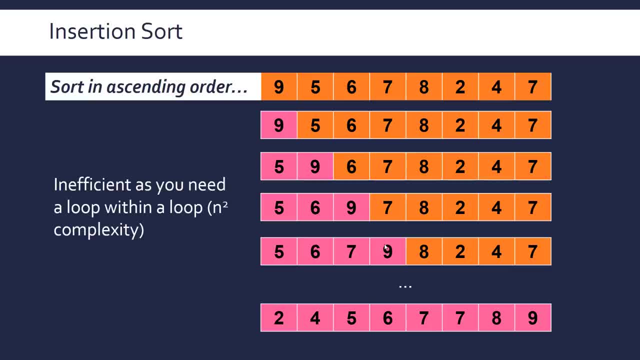 It's hopefully obvious how this works. So it just makes its way through and then loops to compare your element in the sorted part so you can add it, Which is why it's not hugely efficient. So if we look at them, compared all three algorithms, we looked at bubble, sort and insertion. 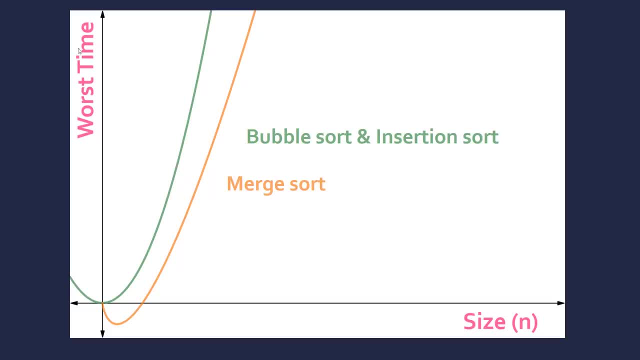 sort have the same. it's called time complexity, so in the worst case they have the same time. This is just, as I say, a mathematical way to analyse it. The graph looks a bit strange. This is a graph of n squared and this is a graph of n log n for merge sort. 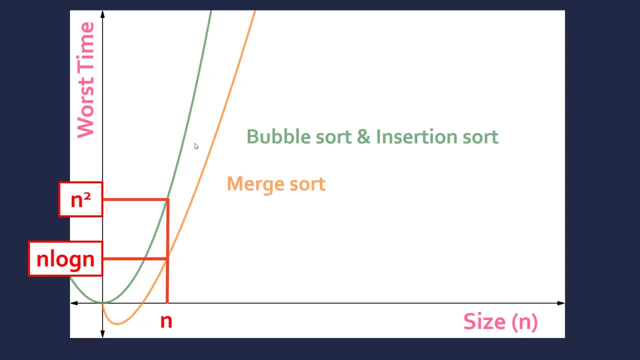 So it's maybe not as clear as with the searching algorithm which one is more efficient. but in the same input size, In the same input size of n, you can see that it takes longer for bubble sort and insertion sort than it does for merge sort in the worst case scenario. 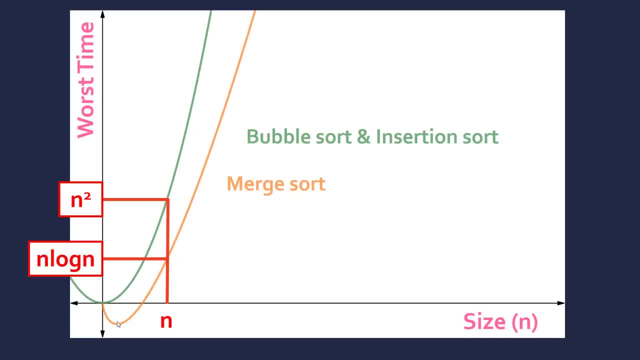 These graphs are slightly strange. The whole idea of analysing it in this way is to just see how the algorithms work as it scales as the input size grows.